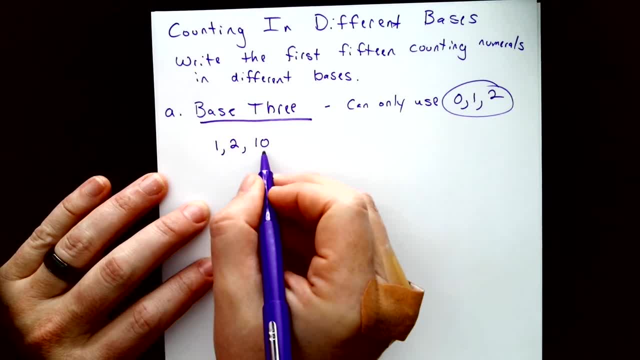 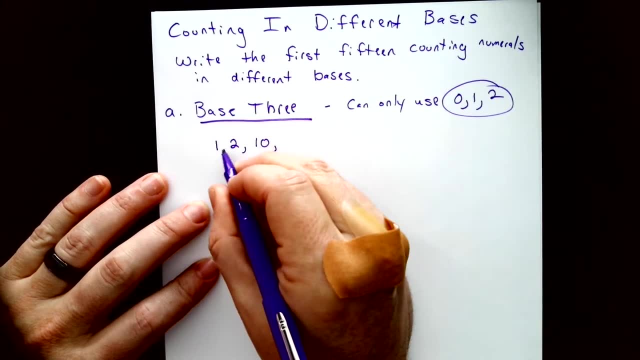 So this is a 1 with a 0 behind it. This is 3, right here. So 1,, 2,, 3.. It looks like a 10.. And then our next one. we would raise this digit up by 1, just like we raised this one up by 1.. 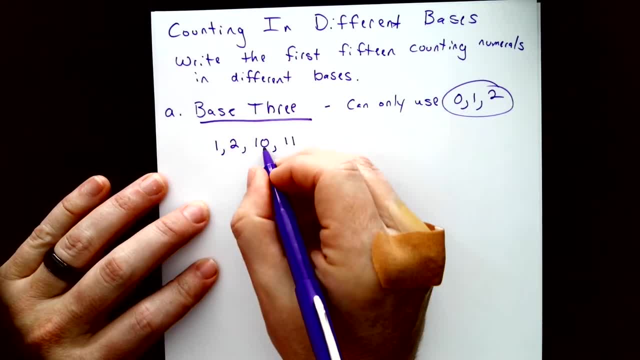 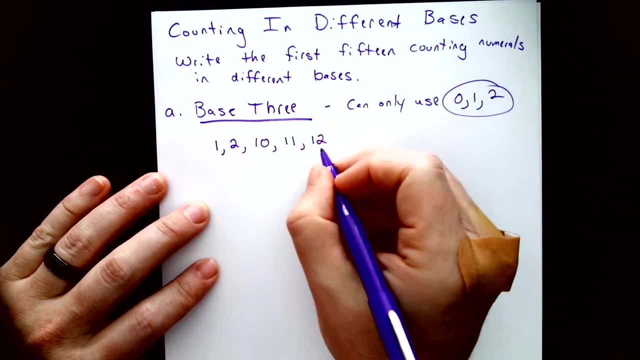 Now we'll raise this digit up by 1, so the next one will be 1, 1, because the 0 goes up by 1. And then the next one would be 1, 2.. Now again, we've completed. 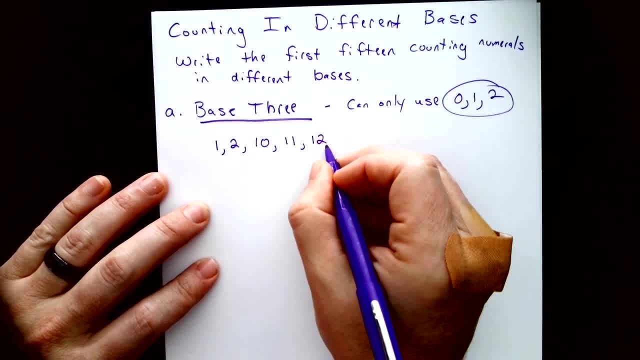 To the same problem that we had before. we can't make this any bigger. We can't say 1, 3, because 3 doesn't exist in base 3.. So we have to raise this digit up again. So we raise that to a 2 and we start over on the digit to the right. 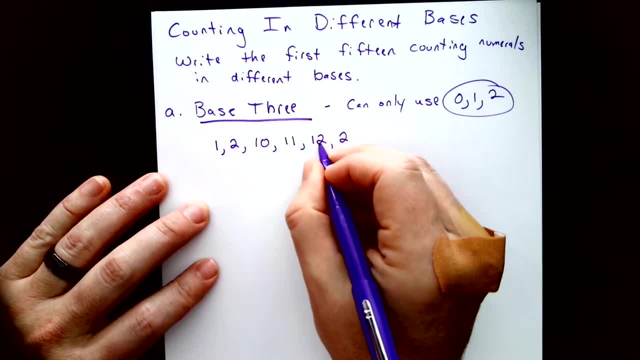 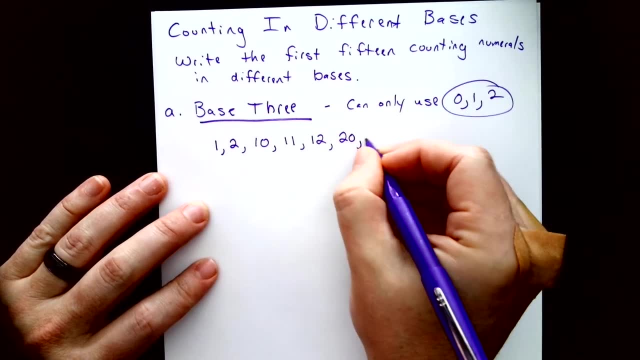 So we go back to 0.. So, instead of saying 2, 2 or whatever, we're going to start over, just like we did 1, 0,, 1, 1,, 1, 2.. Now we're going to do 2, 0,, 2,, 1, and 2, 2.. 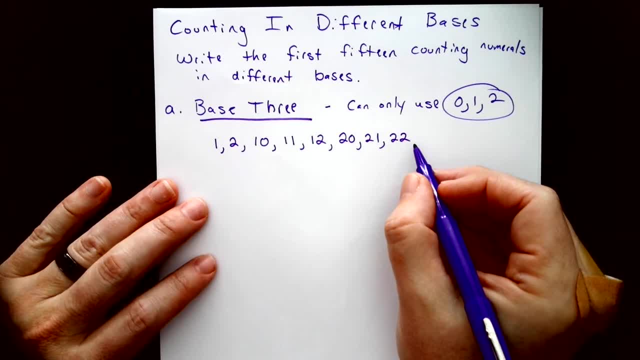 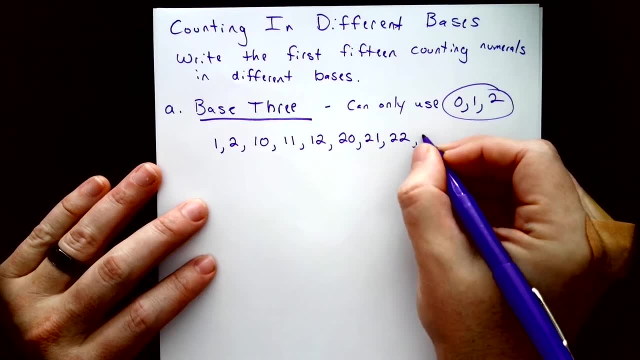 Again, We're back to where we were, in that we cannot put a 3 here, So we're going to have to add another digit over here on the left. We'll make it a 1.. So 1, and then we'll reset these two other digits. 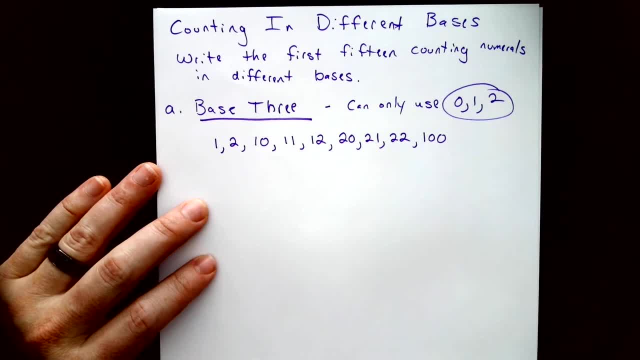 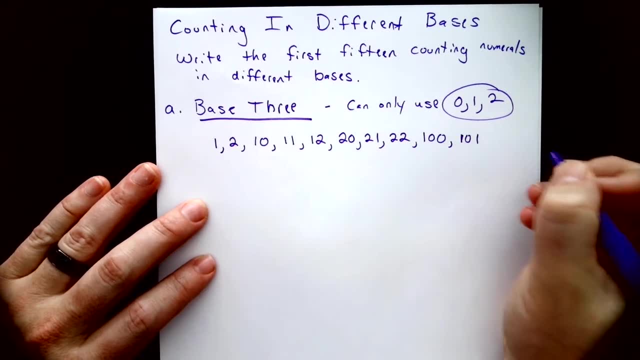 So 1, 0, 0.. In order to get the next one, we start on the right again and we start adding a digit to the right one. So the next one will be 1, 0, 1.. We raise this one up by 1.. 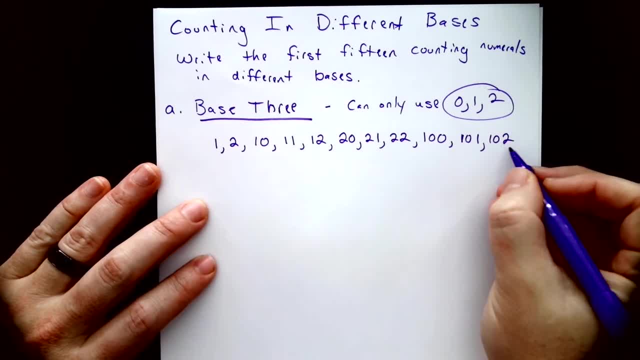 And then it would be 1, 0, 2.. After 1, 0, 2, we cannot put 1, 0, 3, because 3 doesn't exist in base 3. So we have to add a digit here and then reset the one to the right. 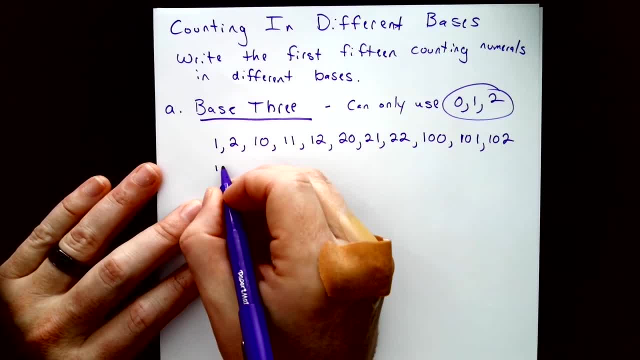 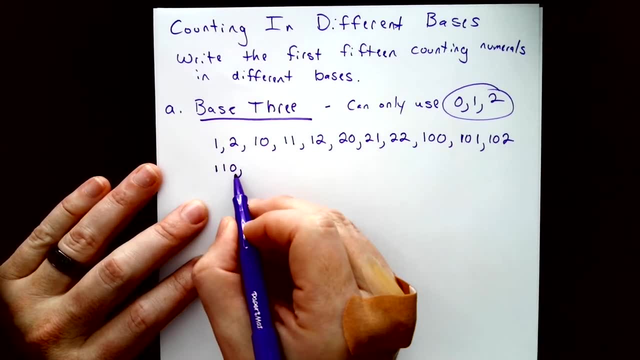 So our next one would not be 1, 0, 3. It would be 1, 1, 0. So we raise this digit up by 1 and then reset it at 0. Then our next one would be 1, 1, 1.. 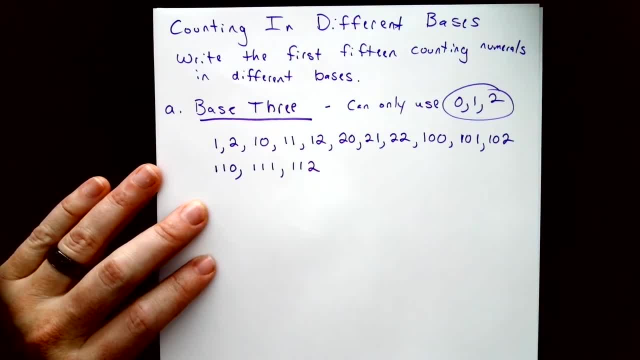 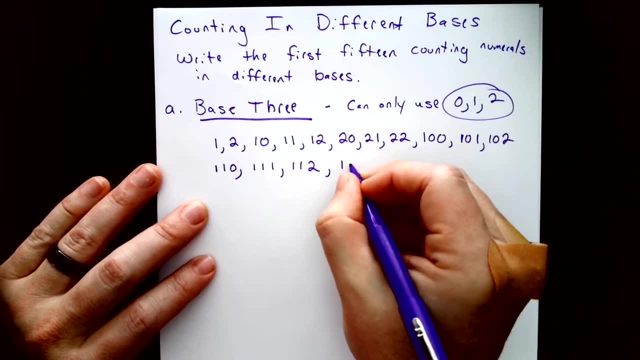 And then 1, 1,, 2. Now we can't put a 3 here, so we have to raise this digit up again. So our next one would be 1, 2, 0. And that may be 15 already. 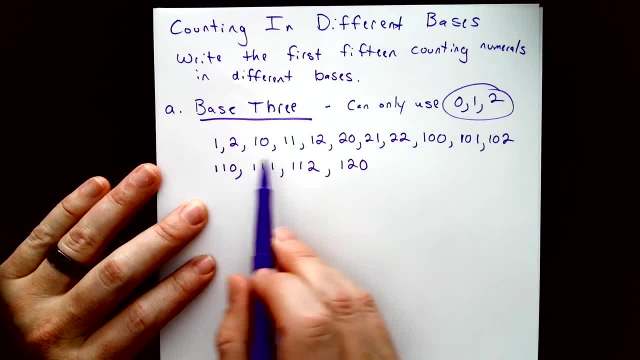 1,, 2,, 3,, 4,, 5,, 6,, 7,, 8,, 9,, 10,, 11,, 12,, 13,, 14, 15.. That's 15.. That would be done. 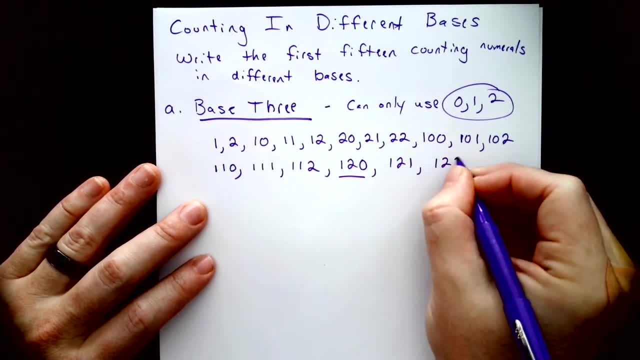 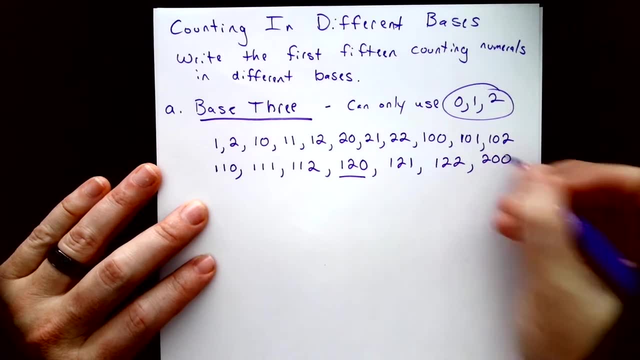 But the next one would be 1, 2, 1.. 1, 2, 2.. And then you've got 2s in both of these digits, so you need to raise it to a 2, 0, 0.. 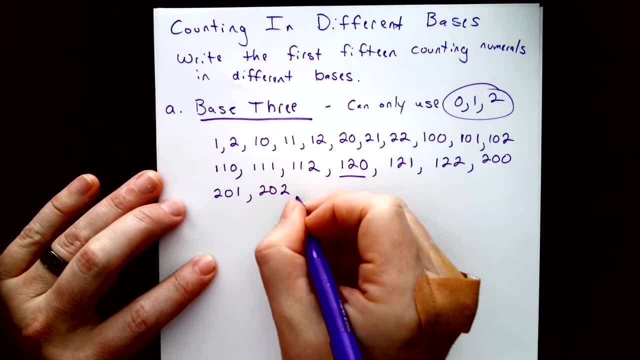 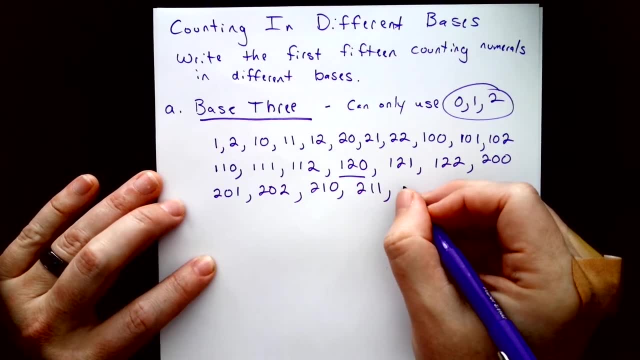 2, 0, 1.. 2, 0, 2.. 2, 1, 0.. 2, 1, 1.. Let's see, The next one would be 2, 2, 0.. 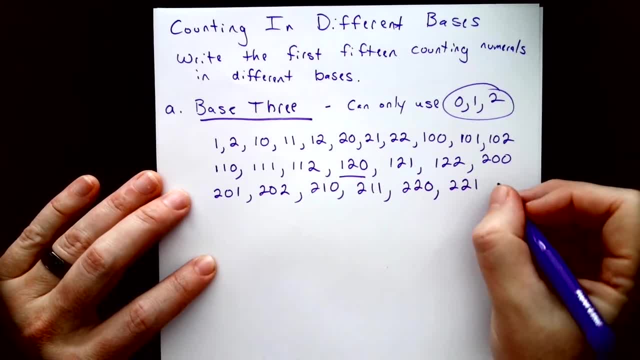 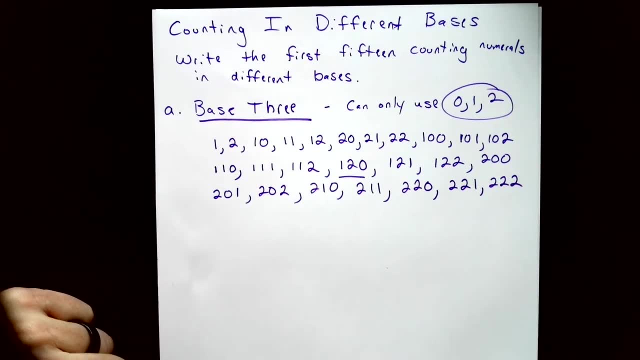 And then 2,, 2,, 1.. And then 2,, 2, 2.. And then you'd have to start again, because you have 2s in all of your digits, Just like we did here. when we had 2s in all of our digits, we had to add a new digit here. 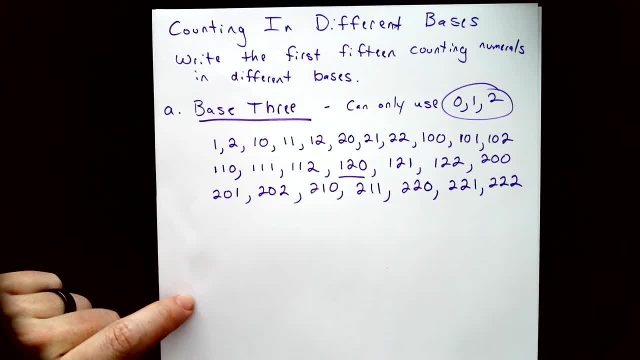 So now, at this point, you'd have to go back to the previous one, You'd have to go to a fourth digit, And I'll do just 1.. It would be 1, 0, 0, 0. And then you'd keep going. 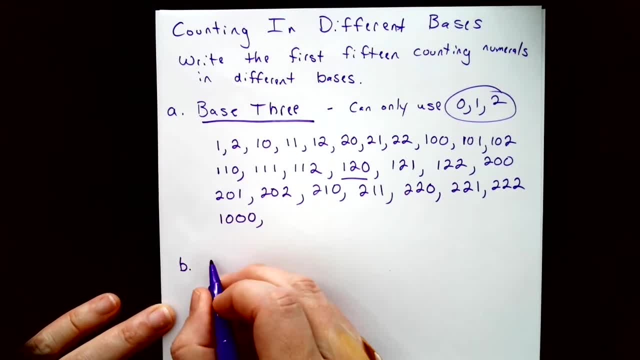 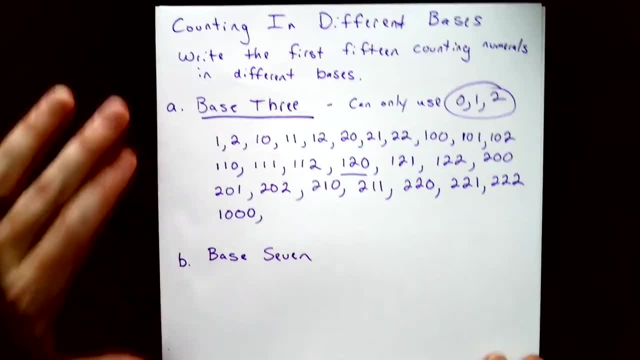 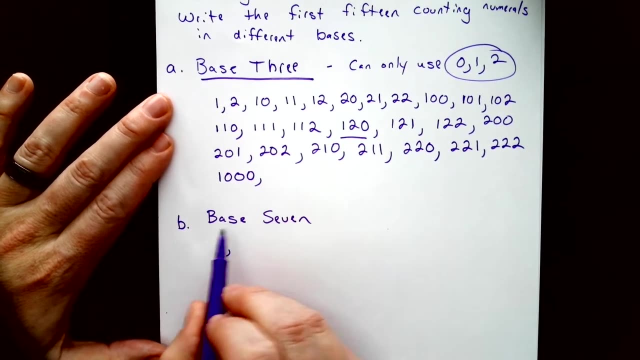 So that's base 3.. Let's do one in base 7.. Let's try to count to 15 in that one as well. So counting numerals again, We'll again start with 1.. And remember we're in base 7, so we can go up to 6.. 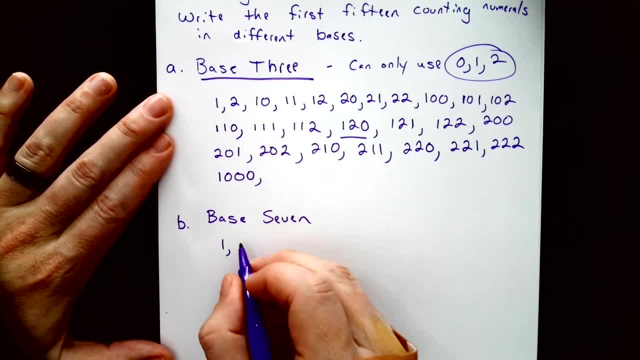 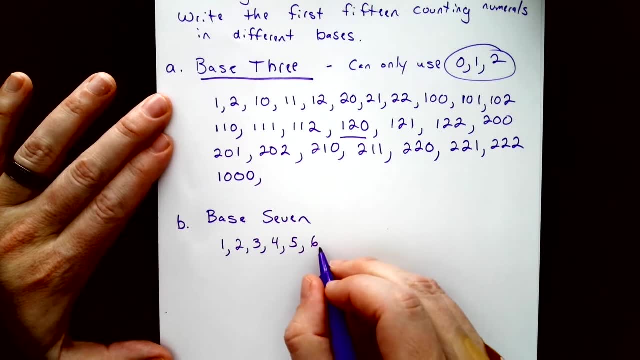 We can't go to 7.. We can go up to 6.. Okay, So we say 2,, 3,, 4,, 5,, 6.. We can't put a 7.. So what did we do up here when we ran out? 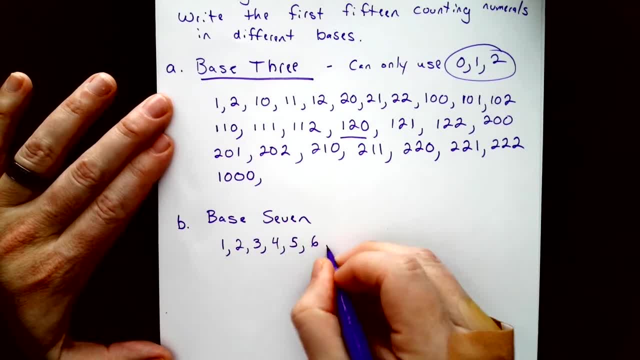 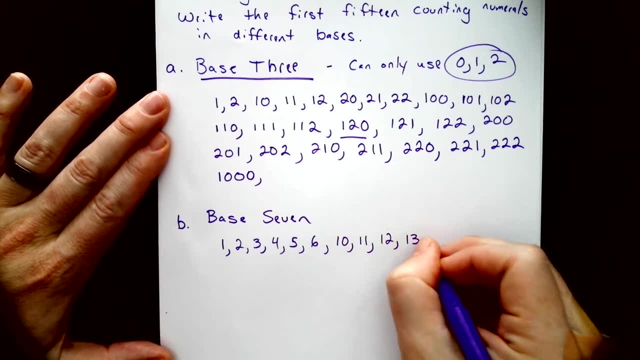 We added another digit. Okay, So we put a 1 and then start at 0.. 1,, 1.. 1,, 2., 1,, 3. 1,, 4. 1,, 5., 1,, 6.. 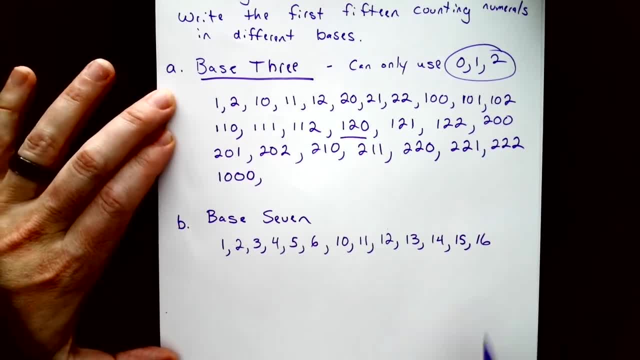 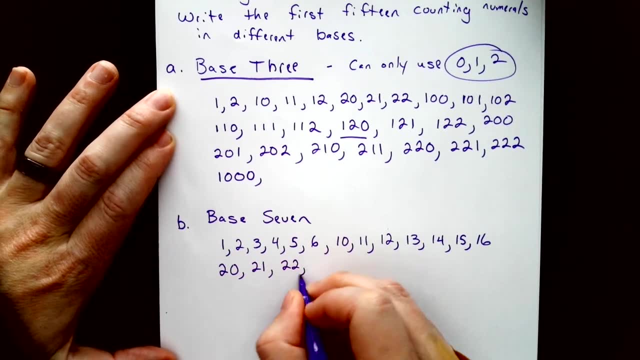 Again, that's as big as we can get. So the next one would have to raise this digit. It's up to 2, 0, 2, 1, 2, 2, 2, 3, 2, 4, 2, 5, 2, 6..